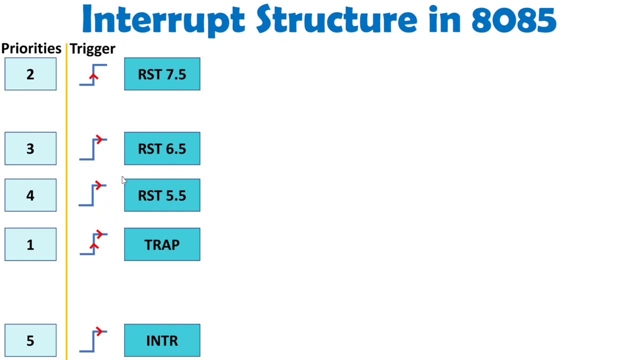 8.5. and INTR, that is getting trigger as per level trigger signal. Now let us try to understand how services will be provided by 8085 whenever interrupt is arising. So first of all I will be talking about INTR, interrupt. So you see, whenever there will be level trigger interrupt. 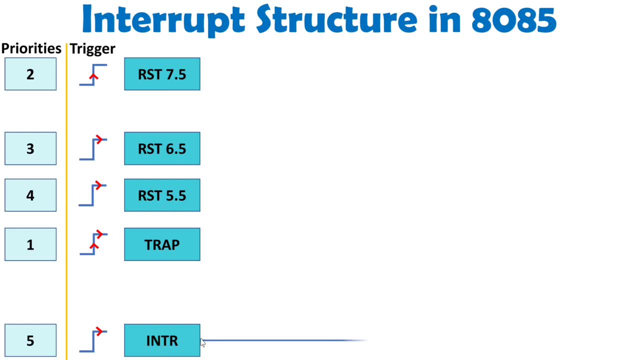 arising from external device with INTR, there will be logic, one which will happen over here, But it doesn't That INTR will get served As INTR is having least priority. there are some other conditions even that we need to see- You will be observing that- to have triggering of INTR. this interrupt. 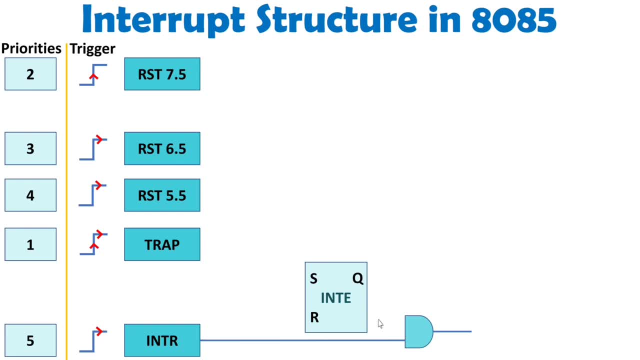 enable flip flop that should give logic one to this AND gate. So whenever this is getting logic one and this is having logic one, at that time there will be interrupt enable with this INTR. right Now this is set: reset flip flop, which is there with interrupt enable. 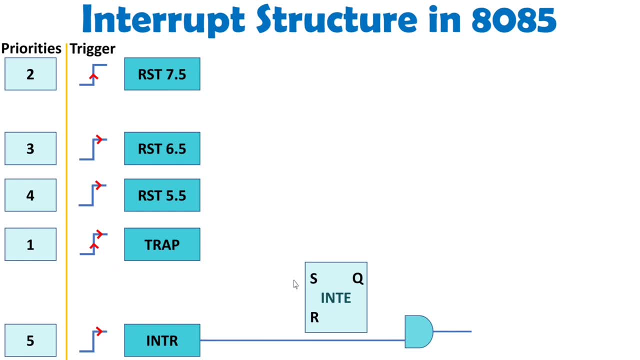 flip flop Now with set. it is very essential that you will have to write interrupt enable. If interrupt enable is executed at set, then only there is a possibility that this Q is equals to 1.. So this is highest priority condition that you must have this set that should have. 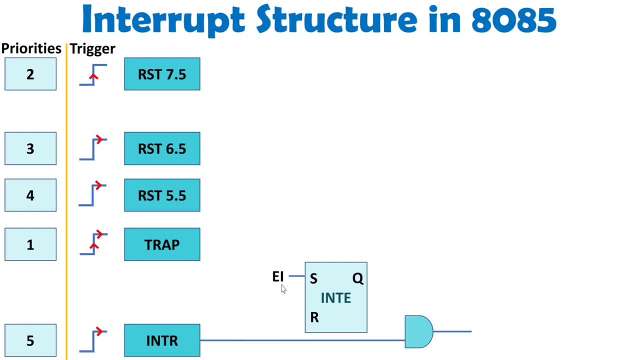 interrupt enable and that should be equals to 1.. So before you complete any other interrupt you will have to enable this interrupt so that next time, whenever another interrupt is arising at that time it will get serve right. So this set reset flip flop is having set terminal that is connected with EI means enable. 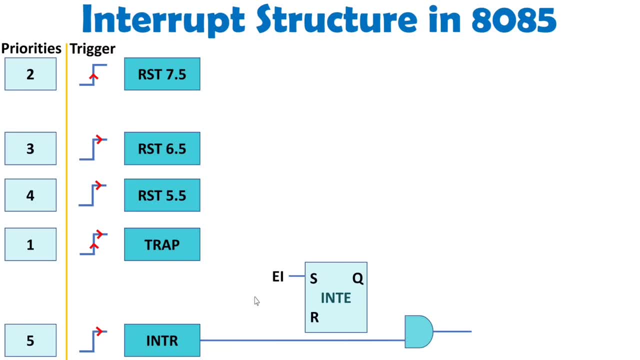 interrupt should get executed, Then only any other interrupt can get service. Now this set terminal that is connected with OR gate and there are many conditions. If DI is there- means disable interrupt is there, then also you will be having reset condition of this INT E flag. If reset is happening, in that case Q will be 0.. Remember this. So this: 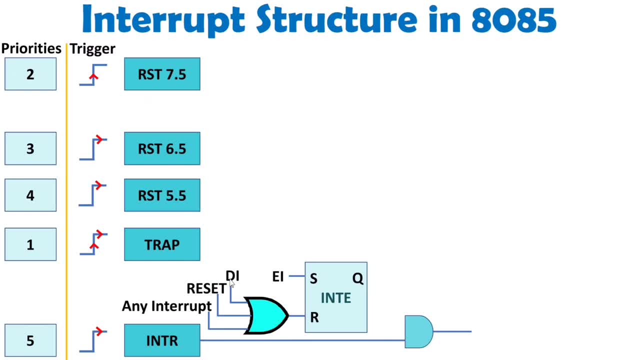 reset. terminal is getting reset by disable interrupt. It can get reset by reset signal as well, as If any other interrupt is arising, then also it will get reset. Why The reason is this: INT R that is having least priority and if any interrupt is having service right now. 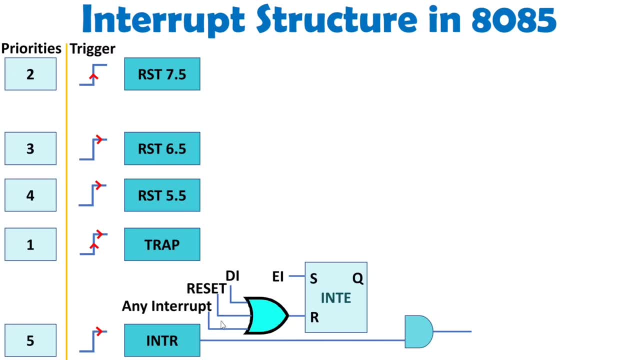 in that case you cannot have service to this interrupt and you will be observing this reset is getting high. So if DI is 1 or reset is 1 or any other interrupt is there, in that case this reset is equals to 1.. So this is the condition. What is the condition? to have Q is equals to 1?. To have Q is equals. 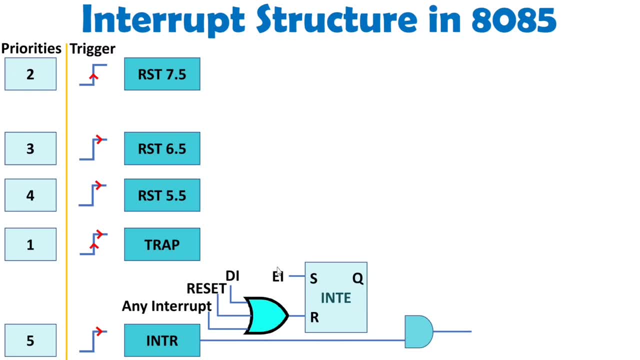 to 1?. What is the condition? This EI that should get enabled, as well as this reset that should be 0, right, As if it is happening, then this Q is equals to 1 and that will make this 11 is equals to one means. now this INT R can get solved Now, as if INT R is having. 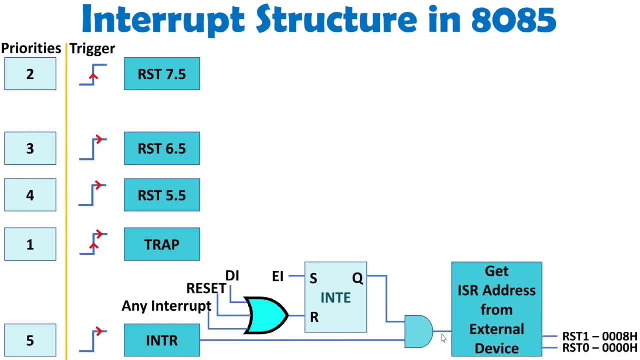 service Right Right now. in that case, what will happen? microprocessor will send interrupt acknowledgement signal to external device and during interrupt acknowledgement, that external device will send any of this rst instruction- rst 0 to rst 7- as if external device is sending rst 0 in that case, 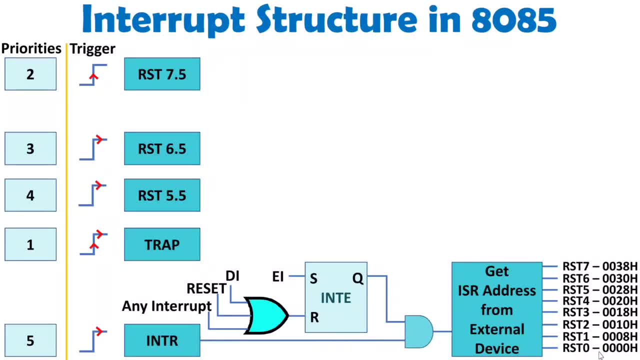 you will be having transfer of control to the location 0 0, 0, 0 hex. if external device sends rst 5. in that case microprocessor will perform interrupt service routine at location 0, 0, 2, 8, hex. so, to remember this, rst 0 to rst 7, my dear students, you should start from 0 0, 0, 0, hex. and 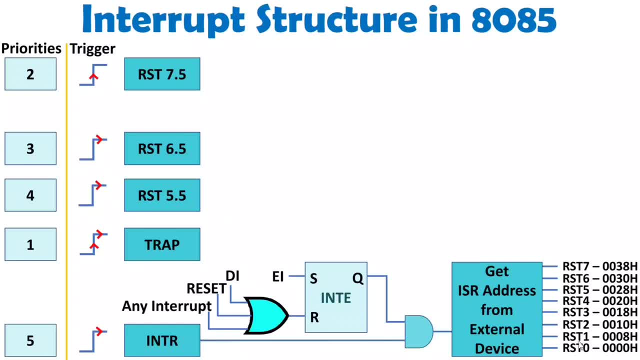 you will have to add 8 when you increment this rst instruction by 1.. right, and that is how you can easily remember these addresses of each of these instructions. so that is how intr is getting executed. now let us talk about trap. so, my dear students, 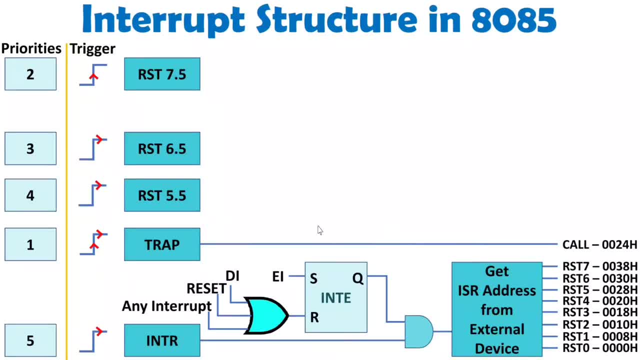 trap is having highest priority and it does not needs any condition. it will get executed immediately once it is identified by 8085. that's why it is age trigger as well as level trigger, as if it is missed by this: 8 0, 8, 5. that's why it is age trigger as well as level trigger, as if it is missed by this. 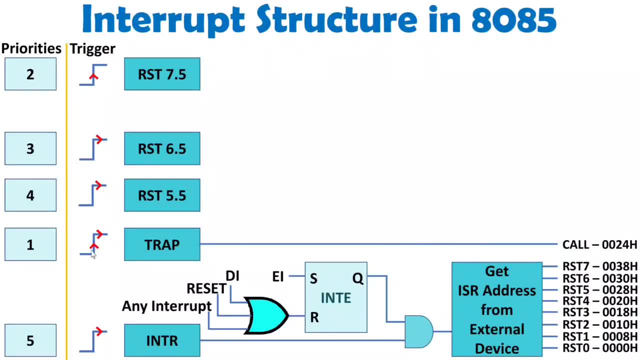 8, 0, 8, 5. that's why it is age trigger as well as level trigger, as if it is missed by this age, in that case by level it will get identified. that's why age and level both are given with this trap and whenever trap is arising, at that time this call will get executed and 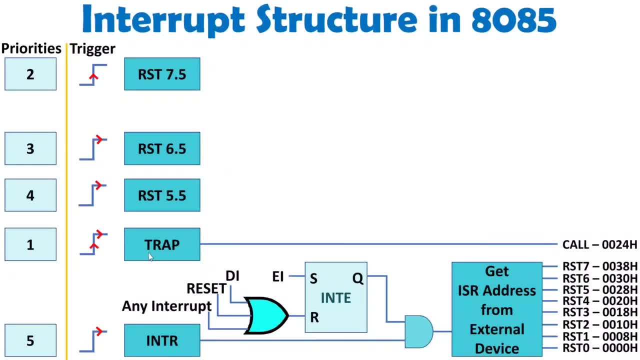 how to remember this address. so, my dear students, initially trap was named as rst, 4.5, and 4.5 into 8, that will be 36, and 36 in terms of hex it will be 0, 0 to 4 hex. that is how you. 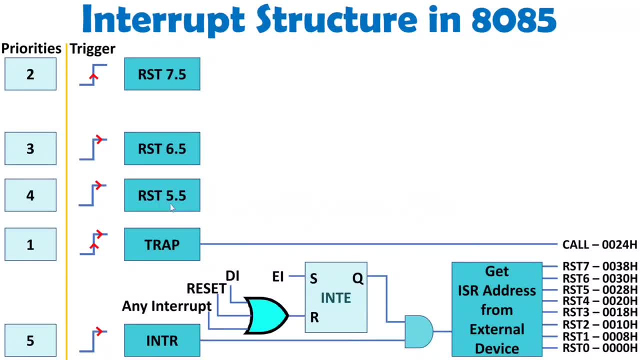 can remember addresses. you can even remember rst 5.5, 6.5 and 7.5 as per. just multiply 5.5 with 8, you will be having address in terms of hex. right now, let us talk about rst 5.5. 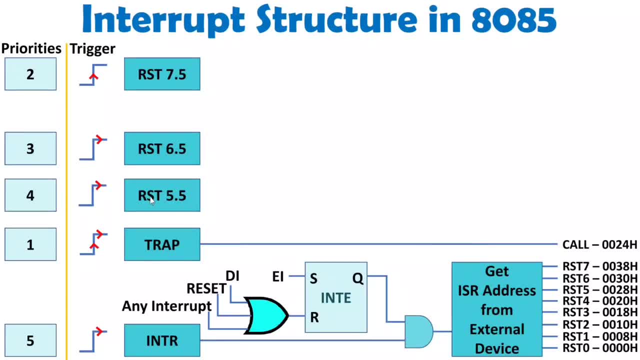 that is having fourth priority. it is level trigger. whenever that is arising here, there will be logic 1, but it cannot get executed immediately. there are some other conditions. even we need to check, like in c instruction. we need to see this bit: m 5.5. it should be 0 in same instruction if m 5.5. 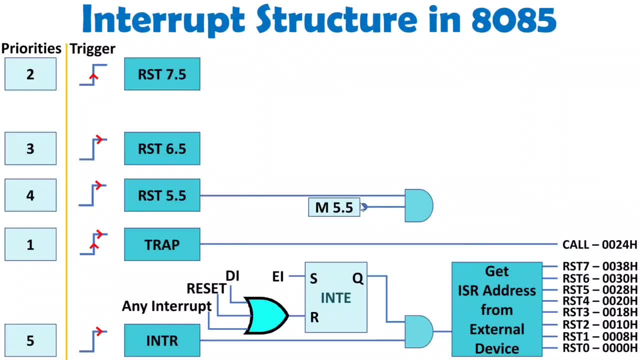 bit is 0. in that case, you see here, bubble is there, so it will make it to 1 over here. so this is one thing that we need to keep in our mind. in same instruction, m, 5.5, that should be 0. right means. you know, don't need to mask it if you write 1, in that case you 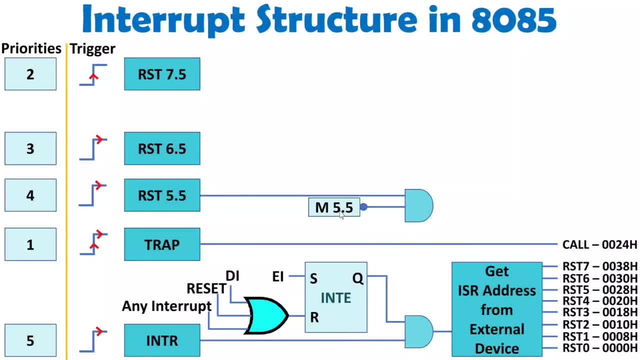 are masking this rst 5.5 as well as one more condition, that is this: q should be equals to 1 over here. so you see, enable interrupt should get executed before you have execution of this. otherwise any of this and get input is 0 then. 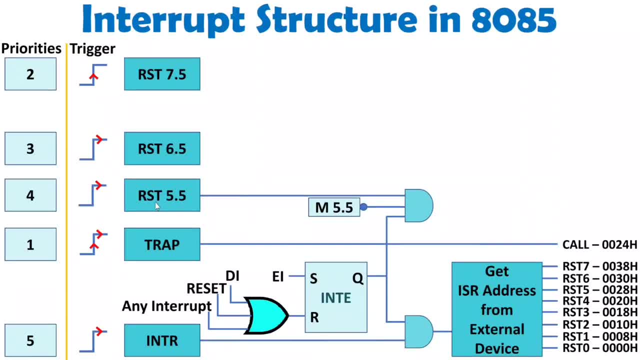 you cannot have output which is performing this rst 5.5 interrupt service. right. once this inputs are 1 over here, there will be call at 0 0 2 c. hex memory 1 over here and if memory location how this is 0 0 2 c, 5.5 into 8, in terms of hex it will be 0 0 2 c. 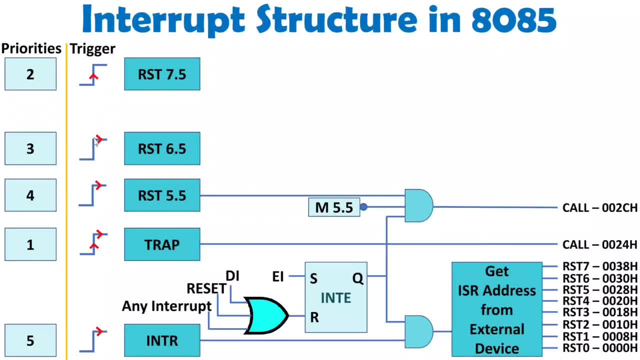 right now. similarly, rst 6.5 is level triggered and when that is getting arised with this and gate, another input should get checked also right, this should be 1 as well as this, same instructions, bit m 6.5.. that should be 0. it should be unmasked. if it is masked, then there will be one. if it is. 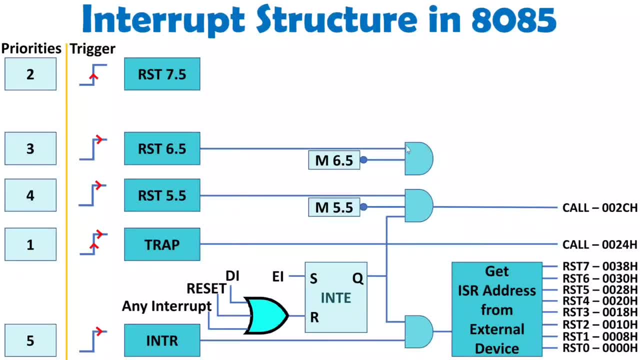 one, then this will be 0. you cannot have one at output of this and gate right, so it is very compulsory this should be equals to 0, so that here after bubble there will be one and this q of this int a that is also connected over here. so if all these three conditions 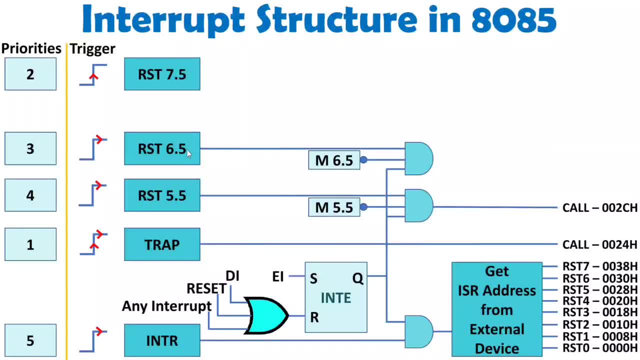 are one over here with this and gate, then rst 6.5 will get served and program control will get jump at 0, 0, 3, 4, hex. and when we talk about rst 7.5, it is age trigger, you see, my dear students. so, as it is age trigger, you will be observing. 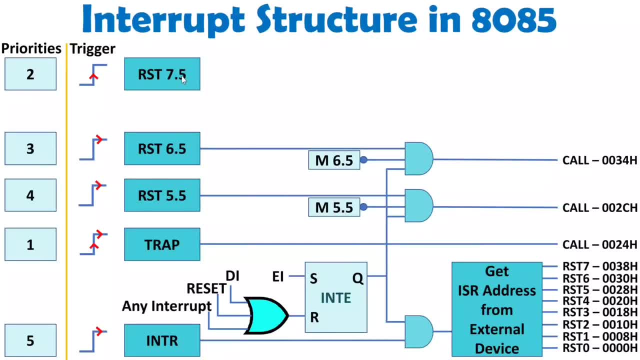 this rst 7.5 that is getting stored inside d flip flop. so here we are having d flip flop and with this d flip flop- As if you are having This Age triggering, this d will get one and that will get translated at output of this q right. 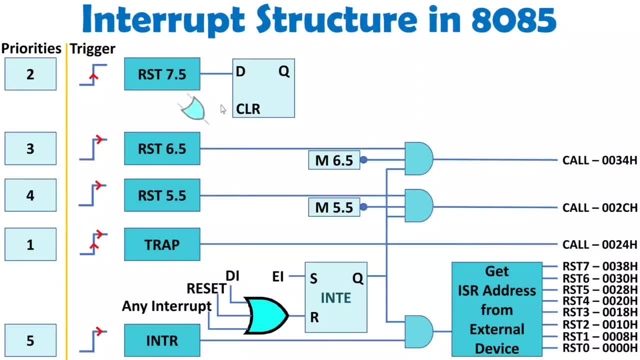 and to clear this d flip flop. there are also some conditions. first condition is: rst 7.5 is recognized. once this rst 7.5 is recognized over here, at that time this clear signal will clear this d flip flop. or to clear this d flip flop, there is one more condition: that 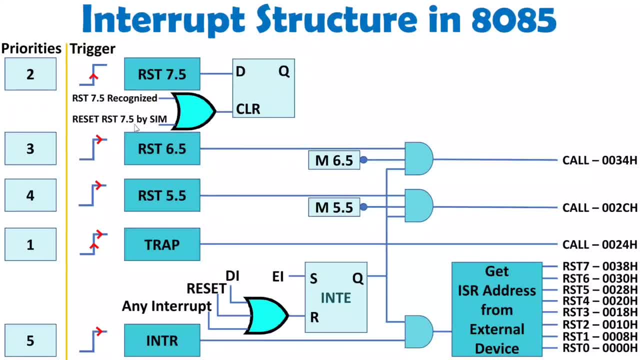 is reset rst 7.5.. By same instruction, so by same instruction. there is a one bit that is reset rst 7.5. in same instruction. I'll explain you how it is getting reset right. so this two condition can clear this flip flop. 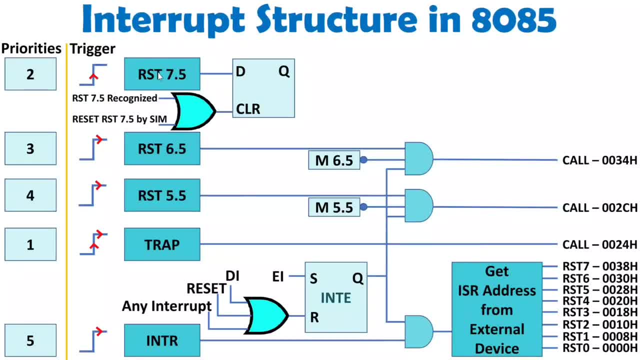 So let us say, here we are having age trigger rst 7.5, this d is getting one and that is getting translated over here. so that is one condition, as well as in same instruction we need to see The masking of 7.5 bit. that should be zero. if it is one, then you can say you have masked. 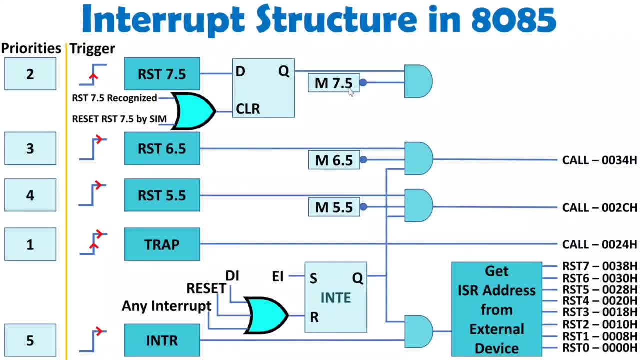 this rst 7.5.. So if it is zero, then after bubble it will be one over here, as well as this q that should be one over here, As if this three conditions are logic one, then you can. so rst 7.5. rst 7.5 can get recognized. 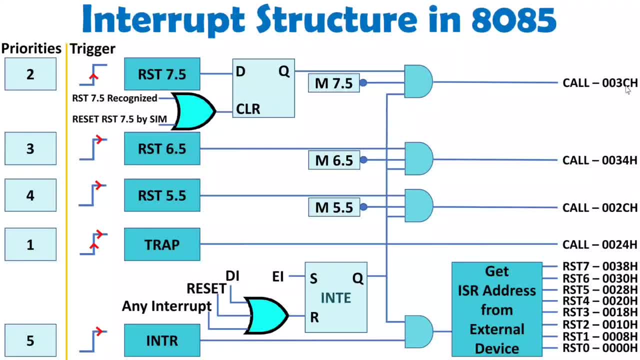 and program control will get transferred to zero, zero, three Hacks. so, my dear students, you should know this. basics first of all. see this: masking can be done with rst 7.5, 6.5 and rst 5.5 trap will be directly connected over here. 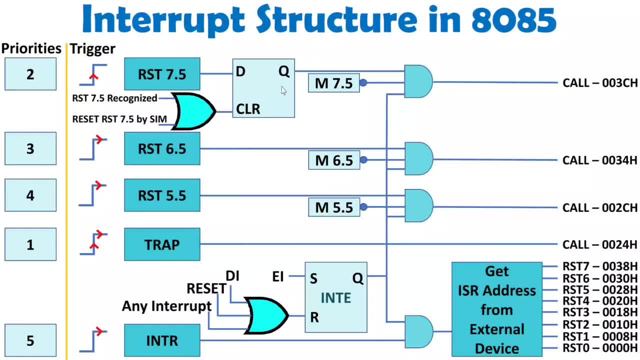 This rst 7.5 that is age trigger, so it will get stored inside this d flip flop. and we need to clear this d flip flop by two possibilities. one is rst 7.5 over here is recognized Okay, And second is by having same instruction. we have reset rst 7.5 by this two ways we can. 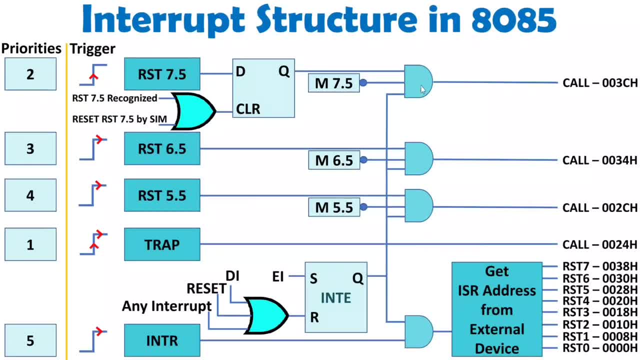 clear this d flip flop and to enable all this interrupts this int flip flop. as per set reset, it should provide logic one over here. to provide logic one: ei should be equals to one and this r should be equals to zero. This r will be zero. 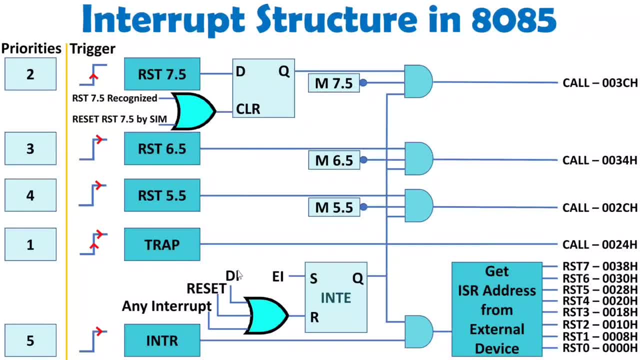 As if So d i reset and any other interrupt is zero. remember this right, And this is what we are connecting it with all the interrupts other than trap right And with i? n t? r. you will be receiving reset instruction from external hardware and then 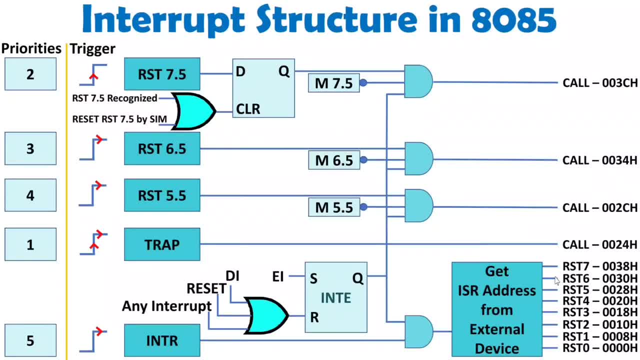 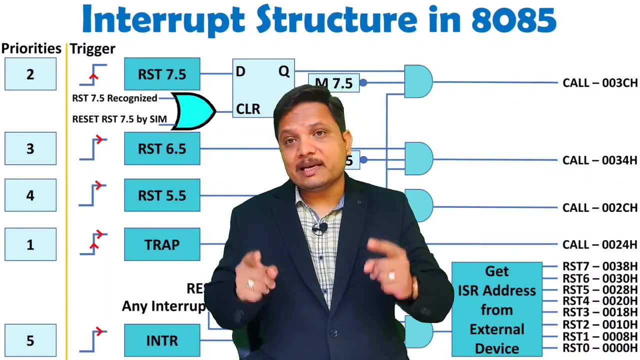 you will be providing transfer of program control for interrupt service routine. But with this hardware interrupt like trap, rst 5.5, 6.5 and 7.5 well defined locations are there. So that is how complete interrupt structure is there. I think now it is clear to you how we can execute any interrupt in microprocessor 8085..